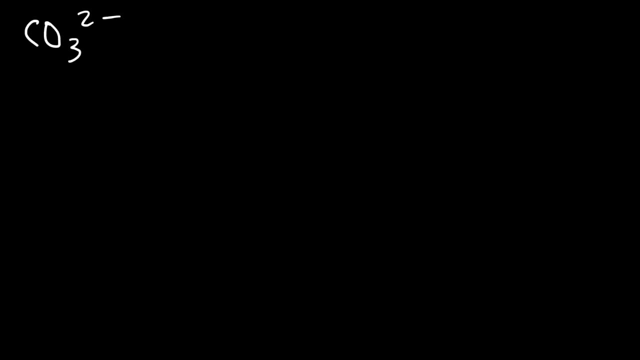 you could find on YouTube somewhere. Now, in order to draw the Lewis structure, we need to add up the valence electrons first. Carbon has four valence electrons and oxygen has six. And don't forget to add two, due to the negative two charge that we have here Now. 3 times 6 is 18 plus 2, that's 20. 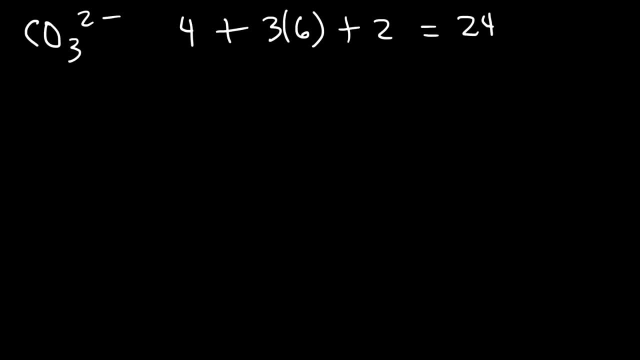 plus the 4, that's 24 valence electrons. Now what I like to do next is I like to calculate the number of lone pairs on the center atom, And there's a formula that I use to do that. It's equal to the. 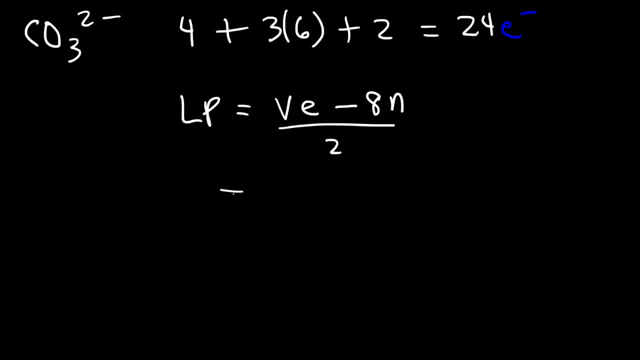 valence electrons minus 8n divided by 2.. So in this example we have 24 valence electrons. n is the number of atoms. That doesn't include the center atom. So we have three non-central atoms, So n is 3.. Now 8 times 3 is: 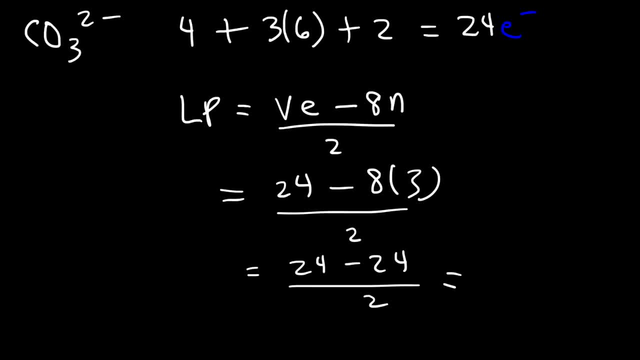 24.. And 24 minus 24 is 0.. So what this means is that there are no lone pairs on the central carbon atom. By the way that equation works, if hydrogen is not present, Carbon likes to form four bonds, And if it's going to be no lone pair, then it's going to have to add up the valence electrons And 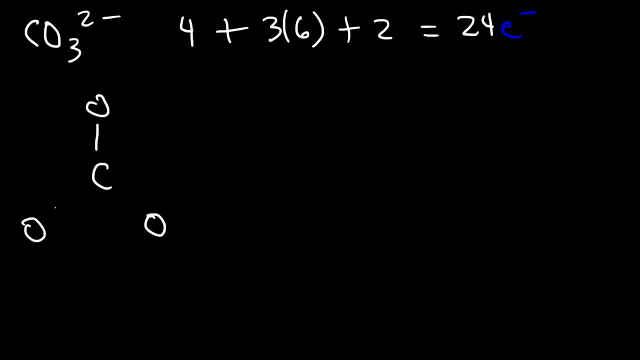 if it's going to be no lone pairs on carbon, we're going to have 1,, 2,, 3, 4.. The last thing that we need to do is fill up the oxygen atoms with electrons. We want every oxygen atom to have. 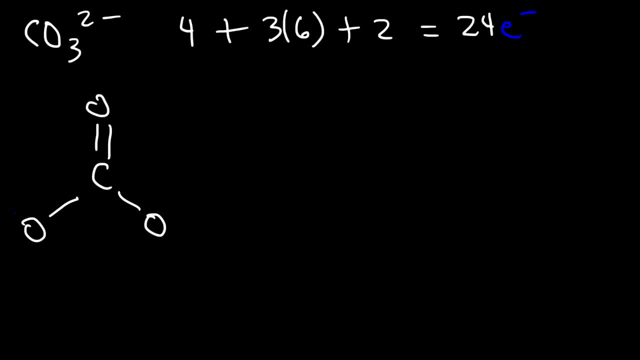 8 electrons. So whenever oxygen has a single bond, we need to add three lone pairs to it, And when it has a double bond, we need to add two lone pairs to it. So this is the Lewis structure of carbonate. Now, whenever oxygen has one bond and three lone pairs, it has a minus charge. Now that we have the Lewis 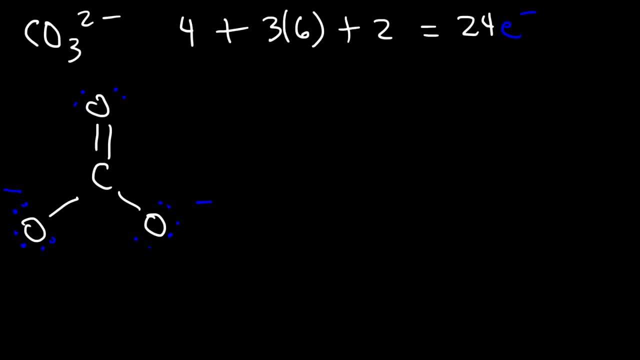 structure of the carbonate ion. how can we draw a resonance structure of it? So notice that some oxygen atoms have single bonds and one has a double bond. To draw the resonance structure, you can move around the double bond among the three oxygen atoms. So what we can do is take a lone pair from this. 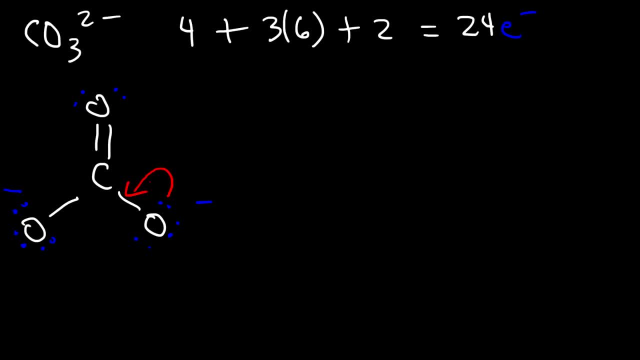 oxygen, Use it to form a non-carbonate atom, Use it to form a double bond. And because carbon can only maintain four bonds, this double bond has to break, pushing two electrons on that oxygen. And so this oxygen here now has a single bond, But this one now has a double bond, So the 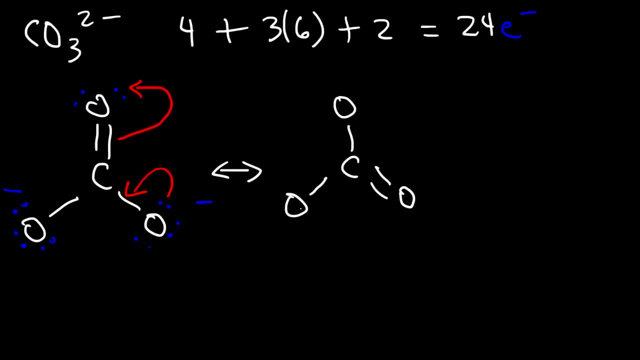 new structure looks like this. So now this oxygen bears a negative charge And the oxygen on the bottom right is now neutral. Now it turns out that we can draw another resonance structure. The third one is this one: We could take a lone pair, use it to form a double bond and cause this pi bond to break. 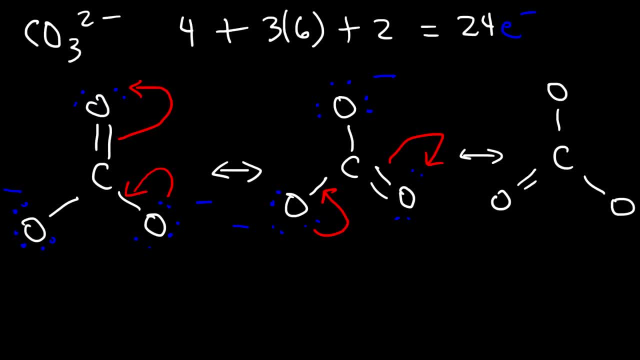 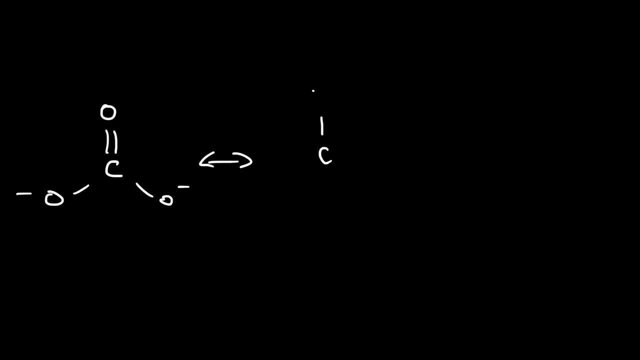 And so now we have this structure. So notice that we can put a negative charge on any one of the three oxygen atoms And all of these three structures. they are equivalent. So I'm going to redraw it without the arrows. So a quick way to show the resonance structures is simply to move the double bond around the. 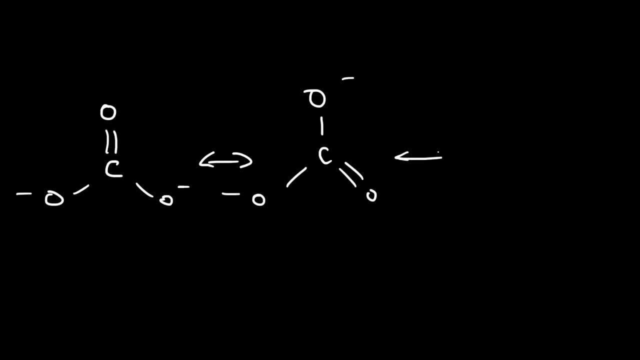 three oxygen atoms. So keep in mind: a resonance structure is simply a way to represent a molecule in different ways. So whenever you want to draw a resonance structure, you need to make sure that the atoms stay where they are. Don't move the atoms. 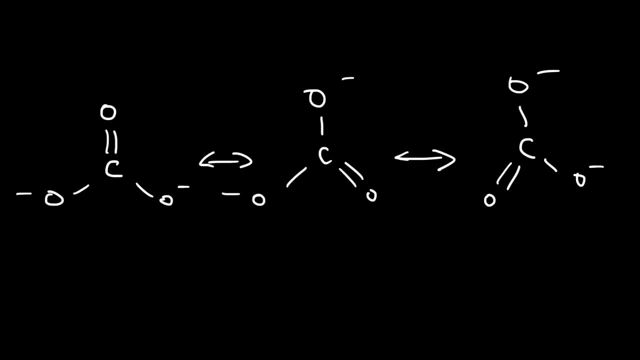 The only thing you should be moving are the electrons. So whenever the electrons move from one spot of the molecule to another, then those two representations are resonance structures. Now the actual molecule is really a hybrid of these three representations, So every oxygen will have at least one bond. 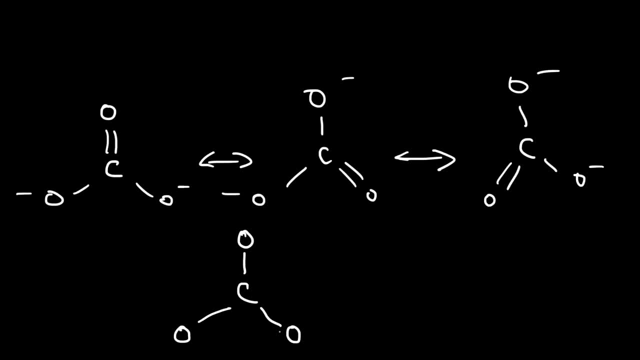 Now the fourth bond. the last bond is actually shared among all three oxygen atoms, So you can represent that with a dash line. So this is the true representation- or this is a better representation- of the actual carbonate molecule. It's a hybrid of these three forms. 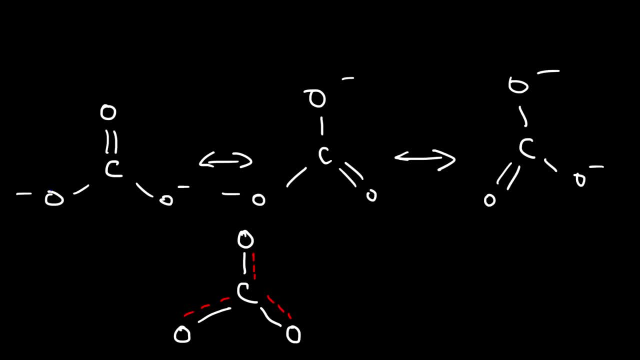 Now, what is the charge on every oxygen atom? Because here it's negative one and here it's zero. The net charge of the carbonate molecule, Or rather the carbonate molecule, The carbonate ion, is negative two, And that negative two charge is shared among three oxygen atoms. 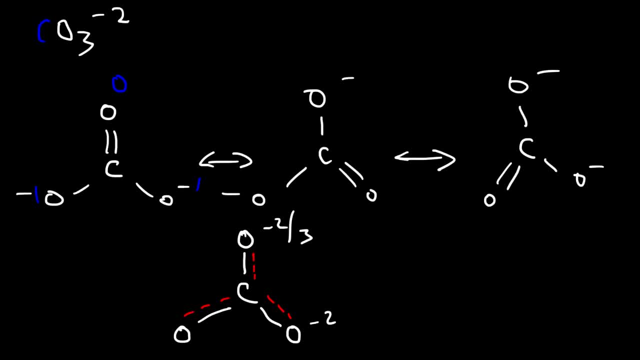 So each oxygen atom has an average charge of negative two thirds. You take the total charge and divide it by the number of oxygens that can bear that charge, And so this is the resonance hybrid of these three resonance structures. So let me give you a practice problem to work on. 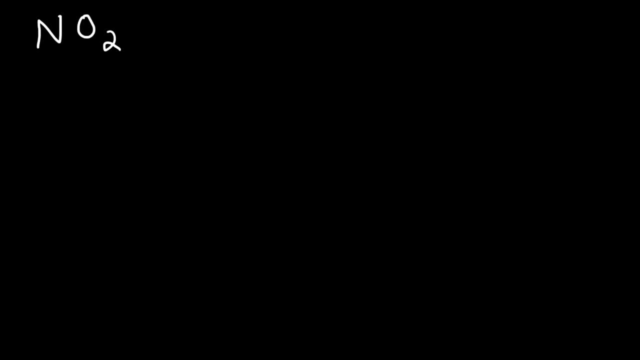 Go ahead and draw the Lewis structure of the nitrate polyatomic ion And then draw all possible resonance structures, including the resonance hybrid. So feel free to pause the video as you work on that example. So let's begin by counting the number of valence electrons. 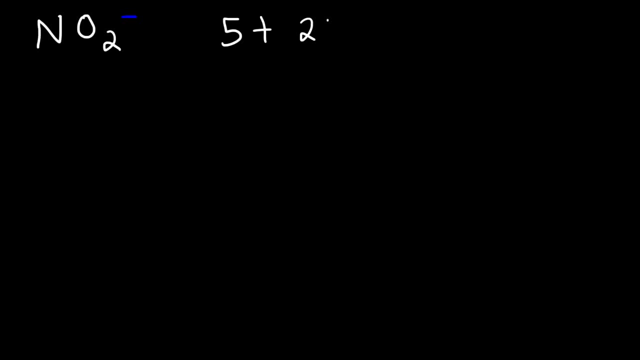 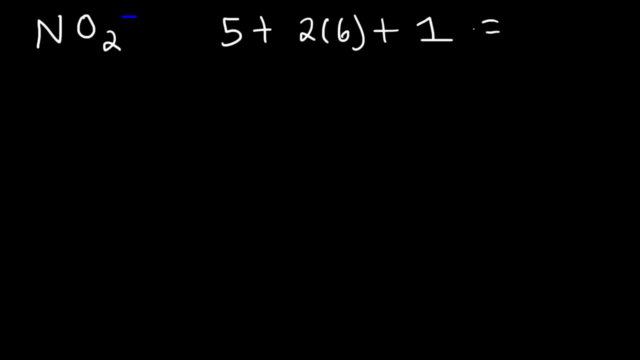 Six times two is twelve plus five, that's seventeen plus one is eighteen, So we have a total of eighteen valence electrons. Next let's calculate the number of lone pairs on the central atom, So that's equal to the number of valence electrons minus 8n divided by two. 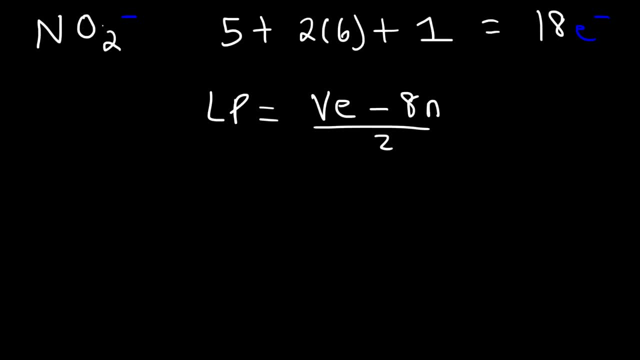 And n is the number of atoms. that is not the center atom, So there's two of those. So we have 18 valence electrons minus 8 times 2 divided by 2.. So 8 times 2 is 16.. And if this number is ever bigger than this number and if you get a negative result, you've done something wrong. 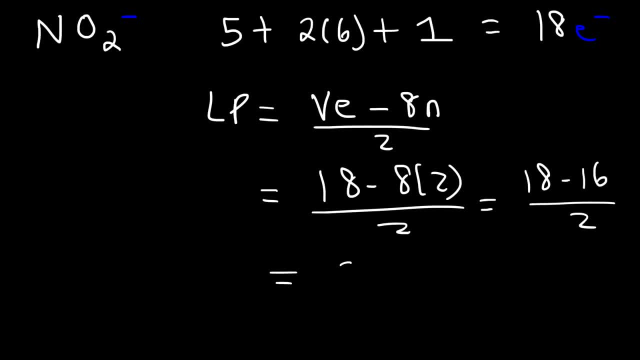 And it's too high. Just so you know, 18 minus 16 is 2.. 2 divided by 2 is 1.. So this tells us that there should be one lone pair on the central nitrogen atom. So I'm going to start with one lone pair on nitrogen. 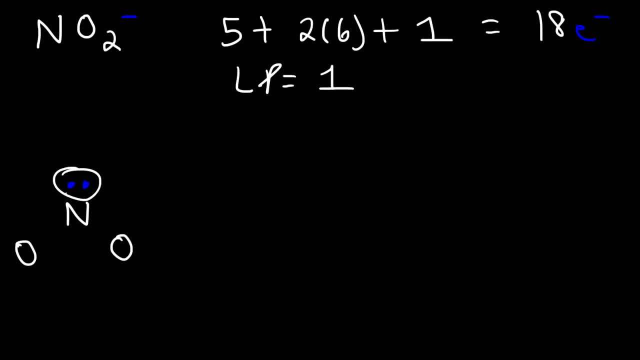 Now nitrogen wants to have 8 electrons. It already has 2. So we need to get up to 8.. This is going to be 4,, 6, and 8. So one of the oxygen atoms have a double bond. 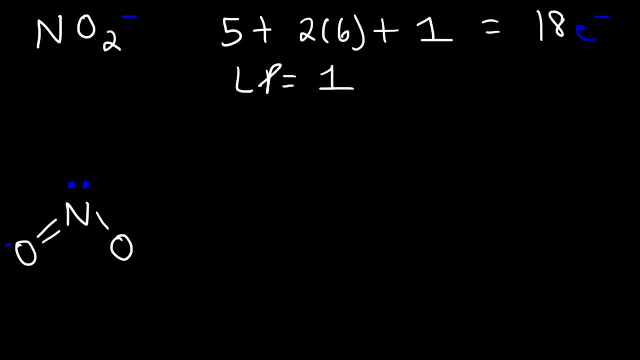 Now we need to fill up the oxygen atoms with lone pairs. So whenever it has a double bond, add 2 lone pairs. When it has a single bond, add 3.. So this is the Lewis structure. If you want to, you could enclose it in brackets.